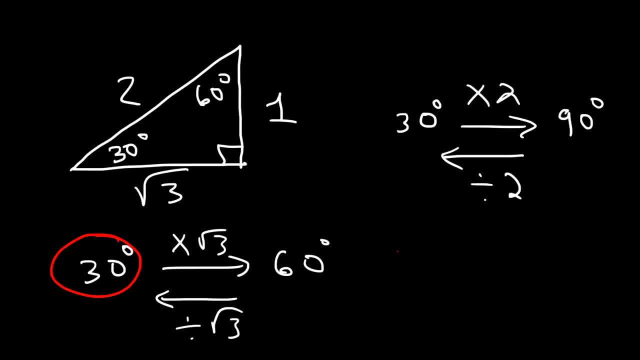 So, if you're going from the side across the smaller angle to the side across a larger angle, you need to multiply. 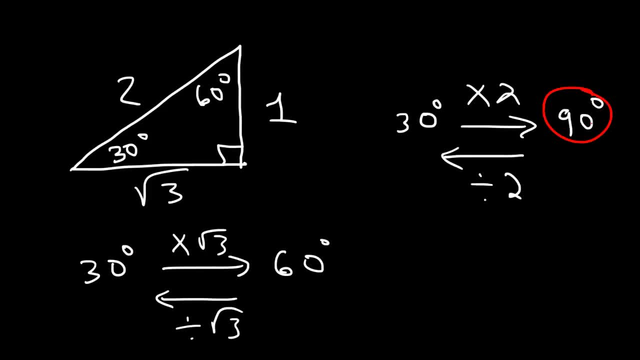 Now, if you're going from the side starting from a large angle to the side across the smaller angle, then you need to divide, because you're looking for a shorter side. 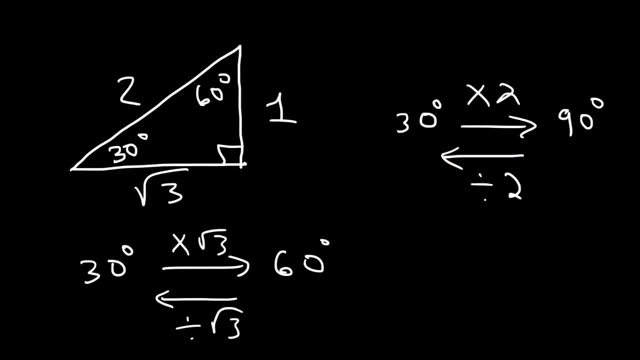 And so, if you're looking for a longer side, longer side, multiply. If you're looking for a shorter side, divide. Now let's put this information 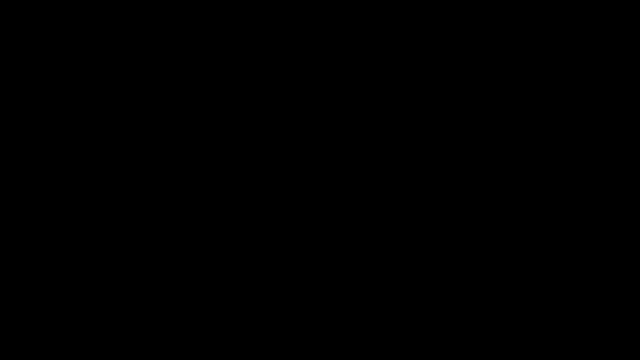 Now let's put this information to good use. So here's the first example. So let's say this is 30 degrees and this is 60, and you know this side is 5 units long. Calculate the length of the other two sides. 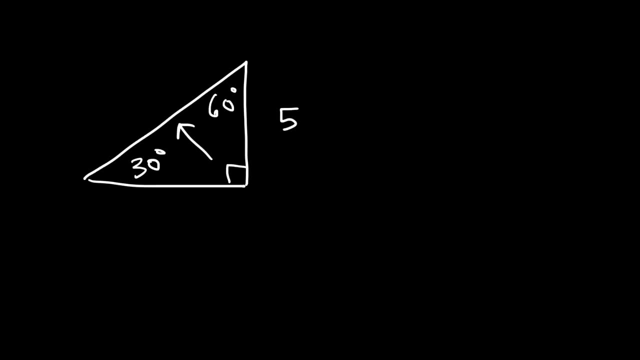 So first let's find the side across the hypotenuse. So we're going from 30 to 90. So we're looking for a longer side. so we've got to multiply And we need to multiply by 2.. 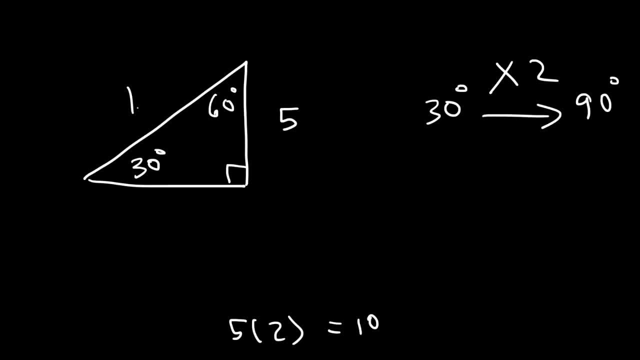 So 5 times 2 is 10.. So the hypotenuse is 10 units long. Now let's go from 30 to 60. You never want to go directly from 60 to 90. Now we're still looking for a longer side, so we need to multiply. 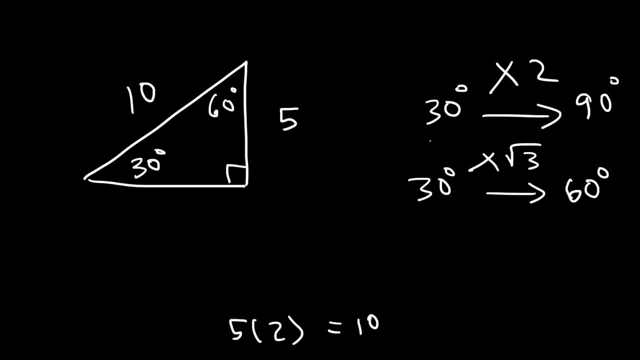 In this case we're going to multiply by the square root of 3.. So it's going to be 5 times the square root of 3, or simply 5 root 3.. And so that's how we could use the 30,, 60,, 90 right triangle to find. 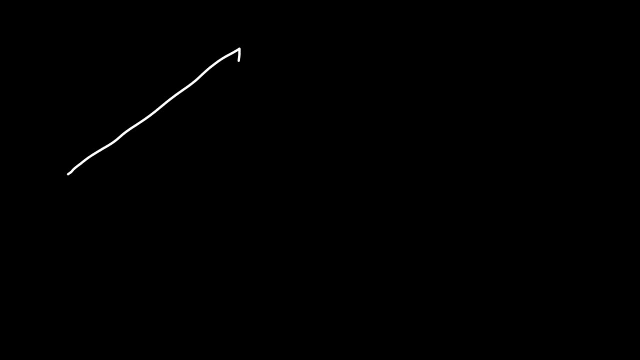 the missing sides. Now let's look at another similar but somewhat different example. So let's say that this side is 12 square root 3. Find the other two missing sides. So let's find the side across the hypotenuse first. 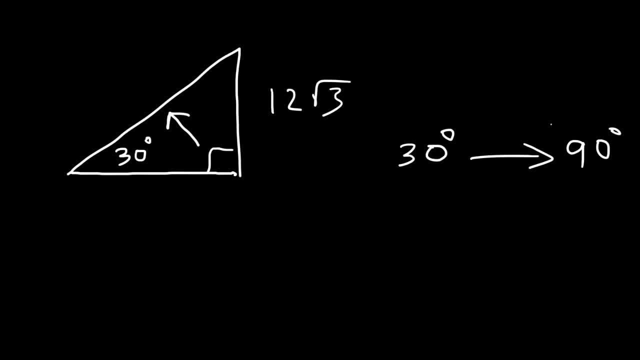 So once again we're going from 30 to 90.. So we need to multiply by 2.. So 12 square root 3 times 2.. We could just do 12 times 2.. This is going to be 24 square root 3.. 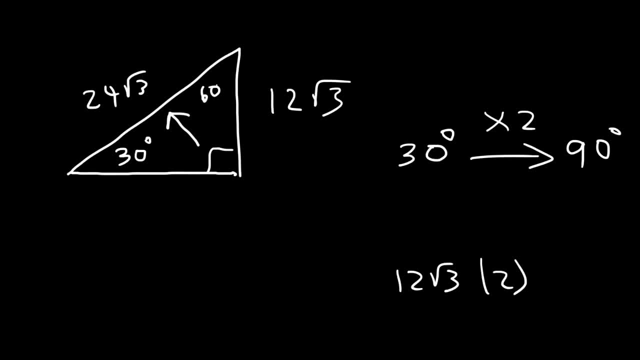 Now we need to find the side across the 60 degree angle. So to go from 30 to 60, we need to multiply by the square root of 3.. So this is the side across the 30 degree angle. 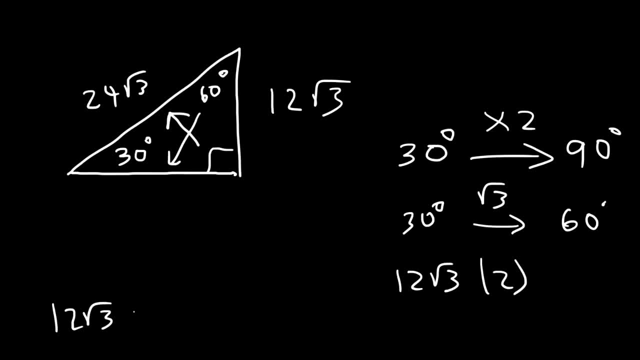 Let's multiply that by square root 3.. The square root of 3 times the square root of 3 is the square root of 9.. And the square root of 9 is 3.. 12 times 3 is 36.. 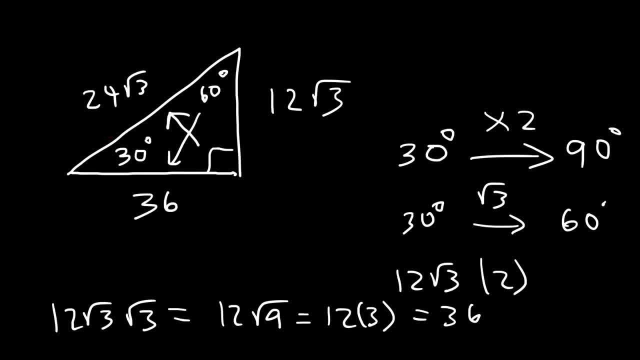 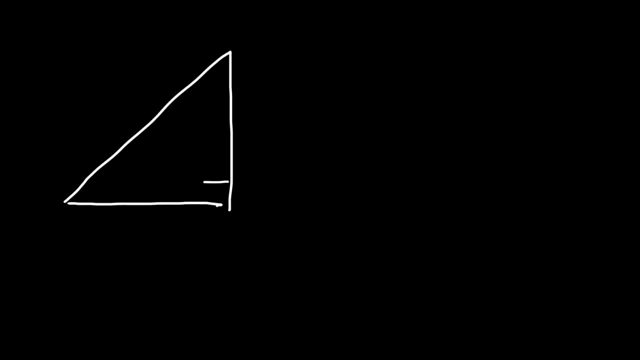 So this side is 36 units long. So that's how we can easily find the two missing sides of the 30-60-90 right triangle, if we know how to use this information. Now here's another example. Let's say that's 12, and this is 60 degrees. 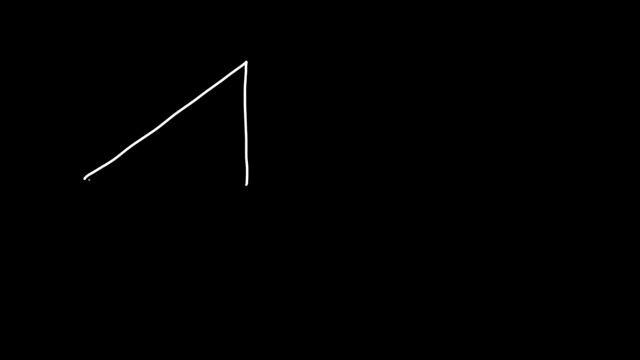 to good use. So here's the first example. So let's say this is 30 degrees and this is 60 and you know this side is five units long. Calculate the length of the other two sides. So first let's find the side across the hypotenuse. So we're going from 30 to 90. So we're looking for a longer side so we got to multiply and we need to multiply by two. So 5 times 2 is 10. So the hypotenuse is 10 units 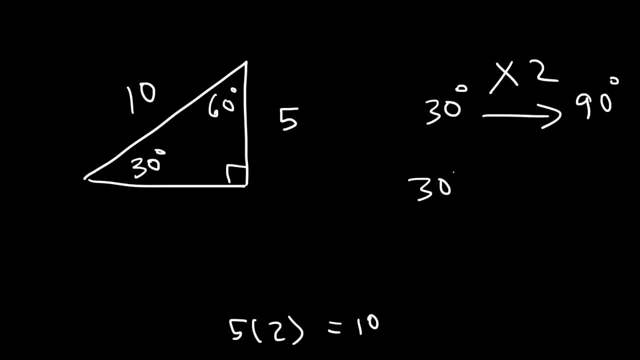 long. Now let's go from 30 to 60. You never want to go directly from 60 to 90. Now we're still looking for a longer side so we need to multiply. In this case we're going to multiply by the square 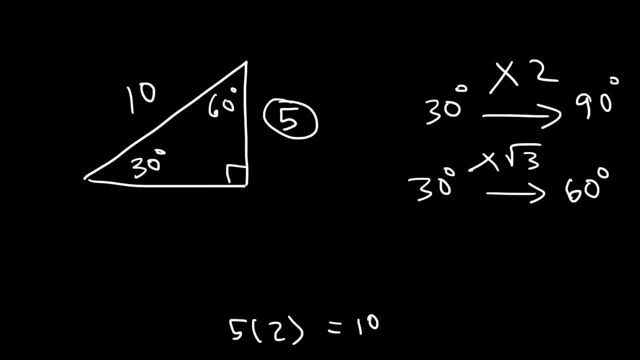 root of 3. So it's going to be 5 times the square root of 3 or simply 5 root 3. And so that's how we could use the 30, 60, 90 right triangle to find the length of the other two sides. 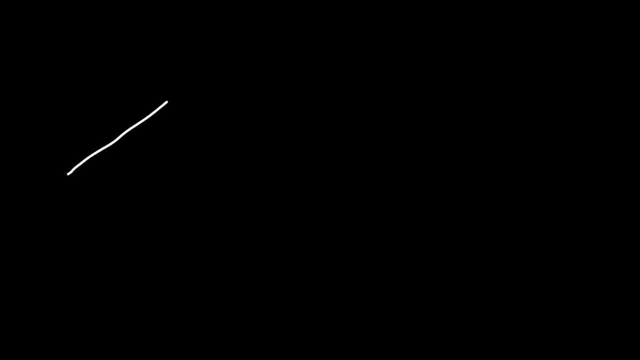 Now let's look at another similar but somewhat different example. So let's say that this side is 12 square root 3. Find the other two missing sides. So let's find a side across the hypotenuse 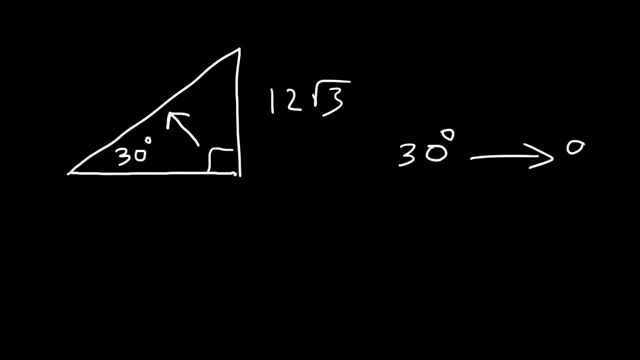 first. So once again we're going from 30 to 90. So we need to multiply by 2. So 12 square root 3 times 2. We could just do 12 times 2. This is going to be 24. 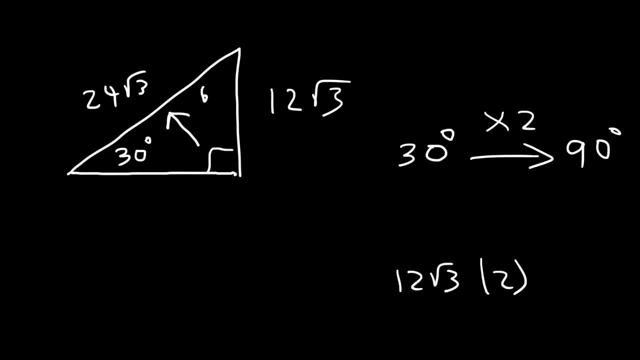 Square root 3. Now we need to find the side across the 60 degree angle. So to go from 30 to 60 we need to multiply by the square root of 3. So this is the side across the 30 degree angle. Let's 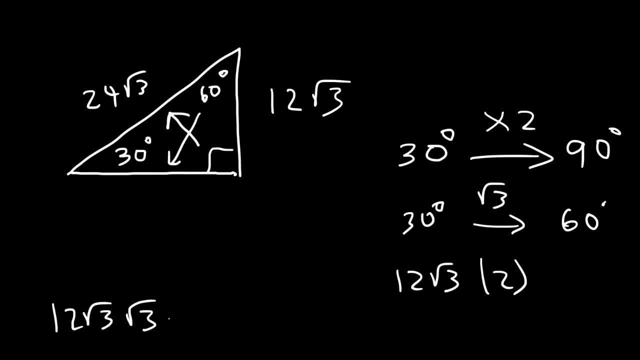 multiply that by square root 3. The square root of 3 times the square root of 3 is the square root of 9. And the square root of 9 is 3. 12 times 3 is 36. So this side is 36 units long. So we need to 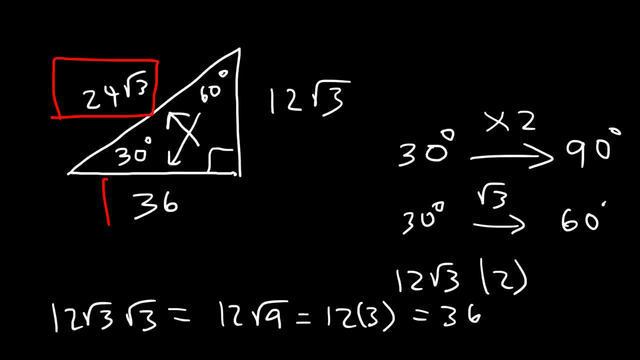 find the side across the 60 degree angle. So that's how we can easily find the two missing sides of the 30, 60, 90 right triangle. If we know how to use this information. 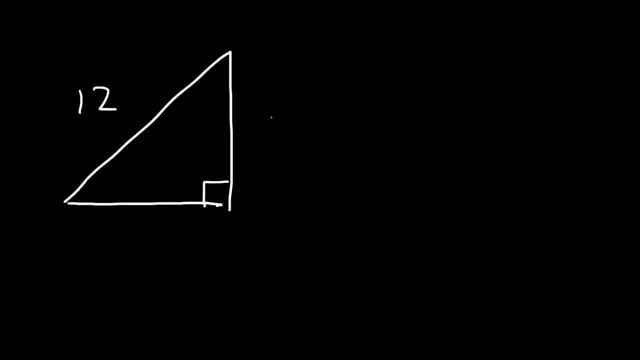 Now here's another example. Let's say that's 12 and this is 60 degrees. Go ahead and find the missing sides. So we know the other angle has to be 30. So this time we're going to find the side 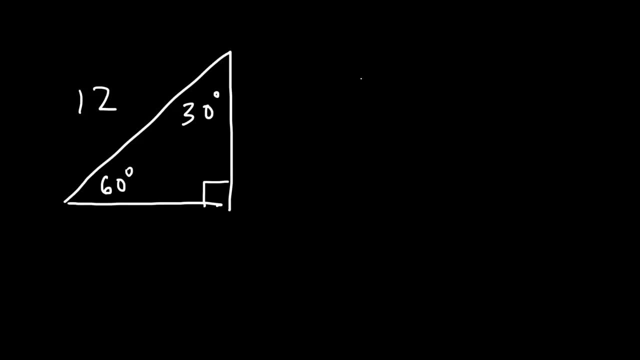 across the 60 degree angle. So let's go ahead and find the missing sides. So we know the other we have the value of the hypotenuse so let's go from 90 to 30 so therefore we need to find the value of a shorter side so we're going to divide instead of multiplying so between 90 and 30 we know the value is 2 so since we're looking 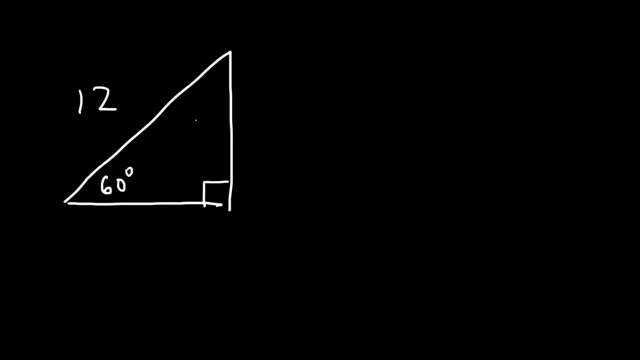 Go ahead and find the missing sides. So we know the other angle has to be 30. So this time we have the value of the hypotenuse, So let's go from 90 to 30. So therefore we need to find the value of the shortest side. 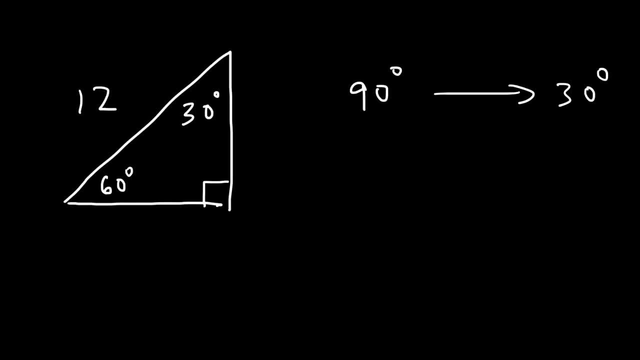 So we've got to divide instead of multiply. So between 90 and 30, we know the value is 2.. So since we're looking for a shortest side, we've got to divide by 2.. So 12 divided by 2 is 6.. 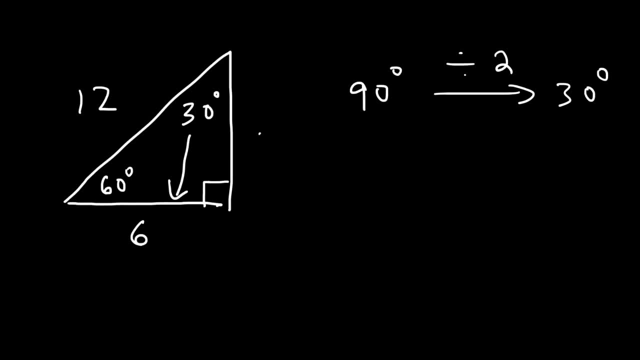 And that's going to be across the 30 degree angle. Now, across the 30 degree angle, we're going to find the value of the hypotenuse. Now, across the 60 degree angle, we need to go from 30 to 60.. 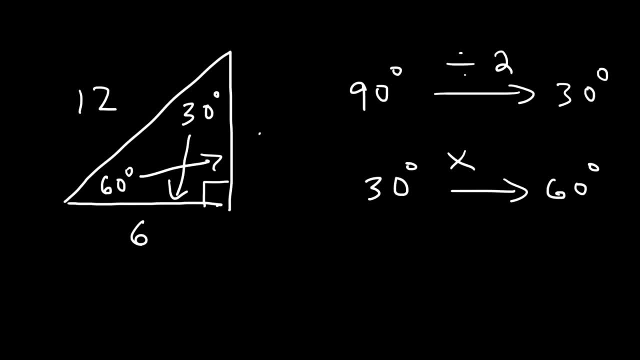 And so we're looking for a longer side. so we're going to have to multiply instead of divide. So whenever you're dealing with 30 and 60, use the square root of 3.. So it's going to be 6 times the square root of 3, which is 6 root 3.. 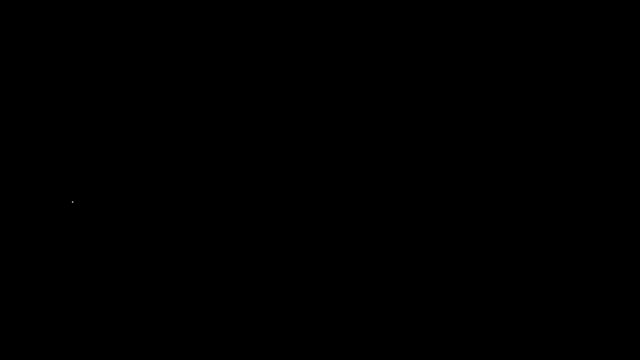 And so that's it. Now let's try another example. So let's say the hypotenuse is 16, square root 3. And this side is 30. Go ahead and calculate the missing sides. So let's go from 90 to 30, because we have the hypotenuse once again. 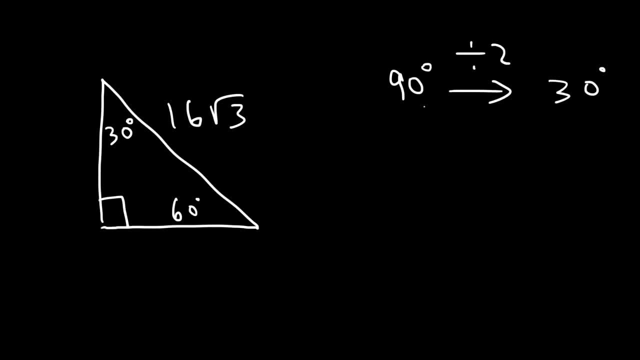 So we're looking for a shortest side. so we're going to have to divide by 2.. 16 divided by 2 is 8.. So across the 30 is going to be 8 square root 3.. Now that we have the side across the 30, we can find the side across the 60.. 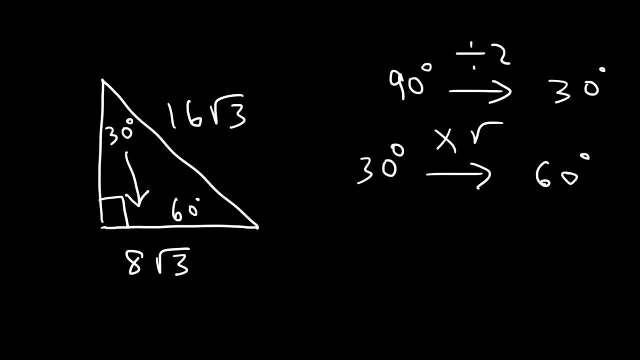 And we're looking for a longer side. so we're going to multiply by the square root of 3.. So this is the side across the 30. So it's going to be 8 square root 3 times the square root 3.. 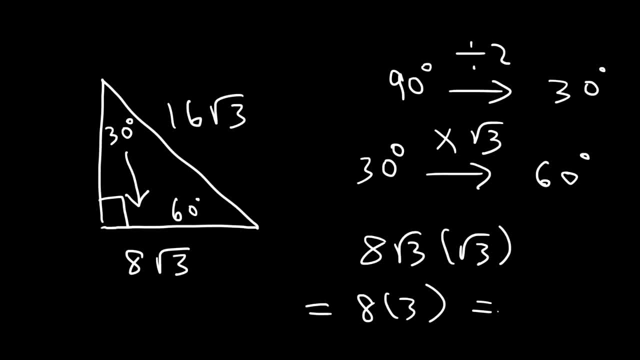 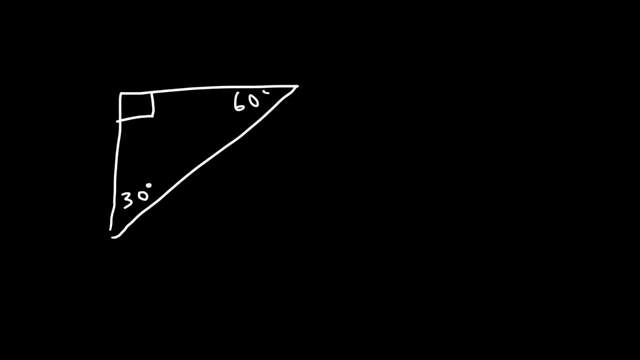 Square root 3 times square root, 3 is 3. And 8 times 3 is 24.. So this side across the 60 is 24 units long. So let's say this is 30 and this is 60.. 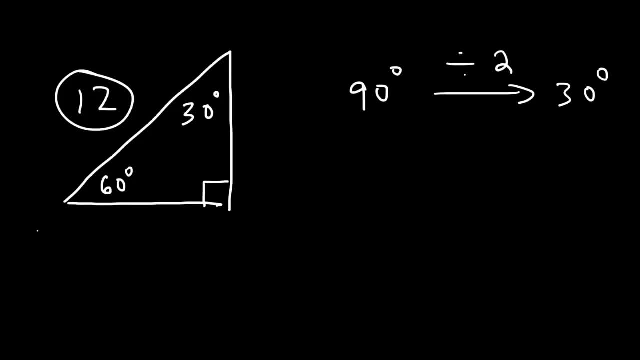 for a shorter side we got to divide by 2 so 12 divided by 2 is 6 and that's going to be across the 30 degree angle now across the 6 degree angle we need to go from 30 to 60 and so we're looking for a longer side so we're going to have to 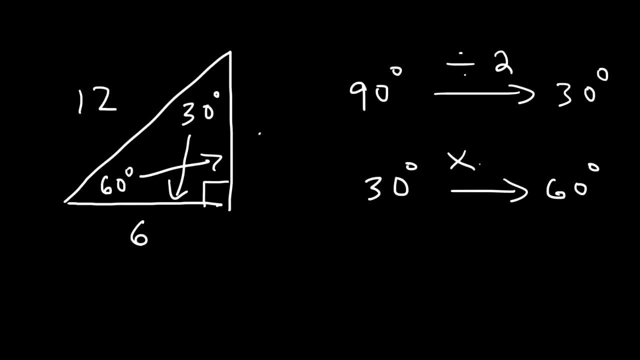 multiply instead of divide so whenever you're dealing with 30 and 60 use the square root of 3 so it's going to be 6 times the square root of 3 which is 6 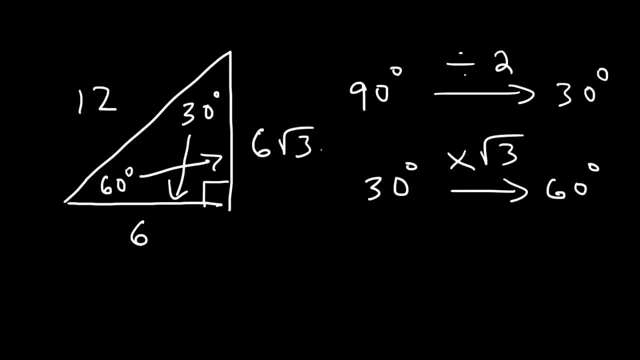 root 3 and so that's it now let's try another example 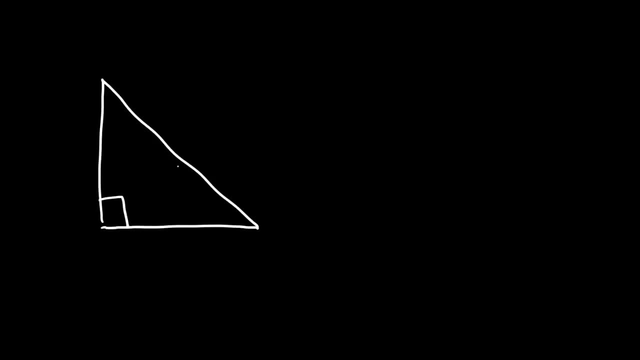 so let's say the hypotenuse is 16 square root 3 and this side is 30 go ahead and calculate the missing sides so let's go from 90 to 30 because we have the 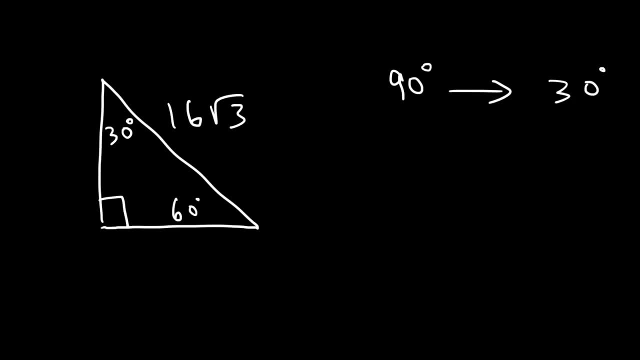 hypotenuse once again so we're looking for a shorter side so we're going to have to divide by 2 16 divided by 2 is 8 so across the 30 is going to be 8 square root 3 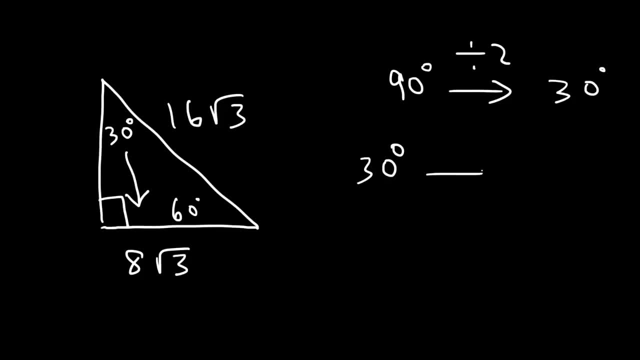 now that we have the side across the 30 we could find the side across the 60 and we're looking for a longer side so we're going to multiply by the square root 3 so this is the side across the 30 so it's going to be 8 square root 3 times the square root 3 square root 3 times square root 3 is 3 and 8 times 3 is 24 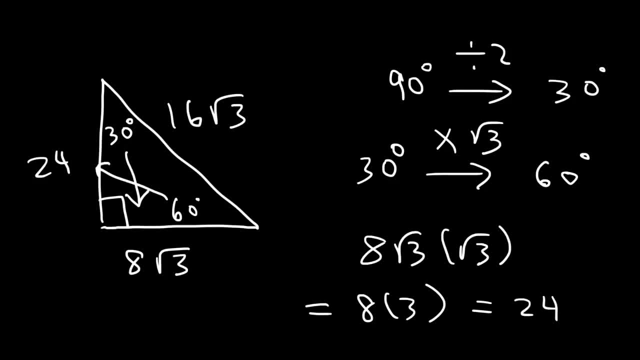 so this side across the 60 is 24 units long 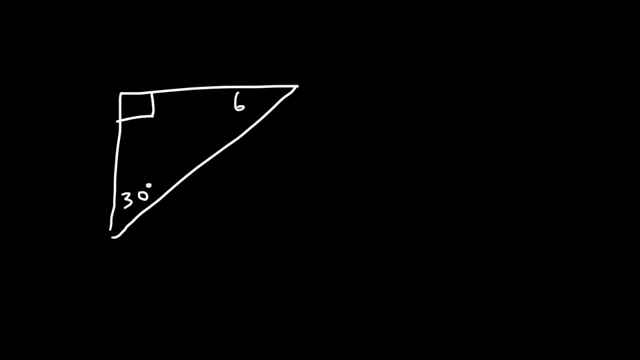 so let's say this is 30 and this is 60 and this time we're going to be given the side across the 60 finding other two sides so you don't want to go from 60 to 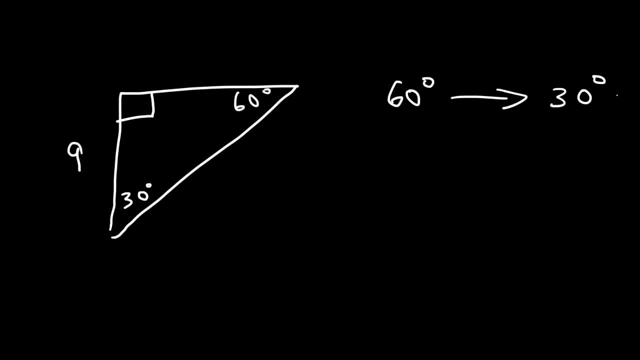 90 instead find a 30-degree side or the side across a 30-degree angle so we're looking for a shorter side so this time we're going to have to divide instead of 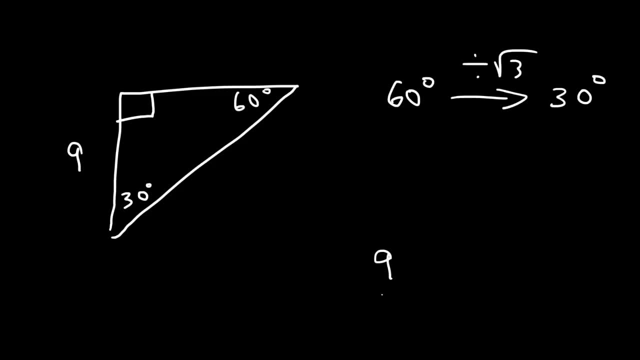 multiplying we're going to divide by the square root of 3 so 9 divided by the square root of 3 we need to rationalize 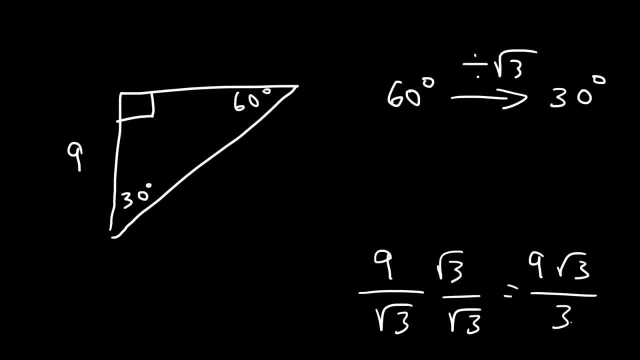 so this is going to be 9 square root 3 divided by 3 and 9 divided by 3 is 3 so 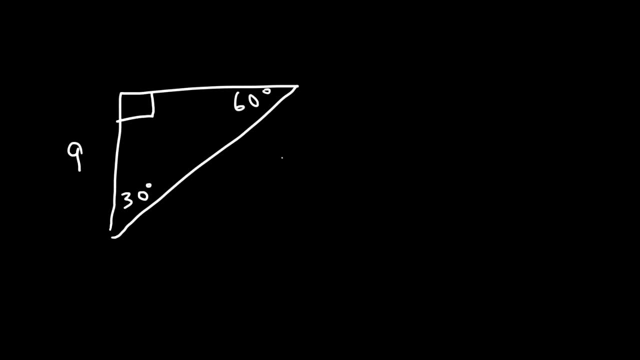 And this time we're going to be given the side across the 60. Find the other two sides, So you don't want to go from 60 to 90. Instead, find the 30 degree side or the side across the 30 degree angle. 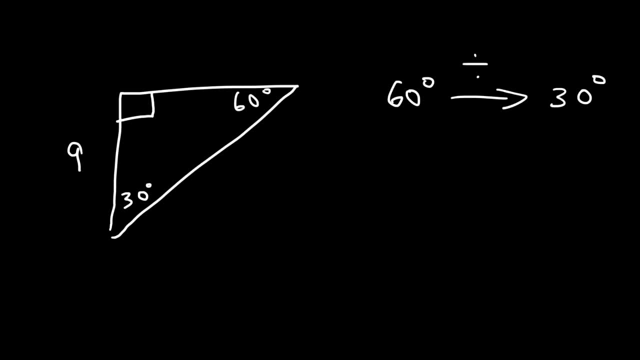 So we're looking for a shorter side. So this time we're going to have to divide instead of multiply. We're going to divide by the square root of 3.. So 9 divided by the square root of 3.. 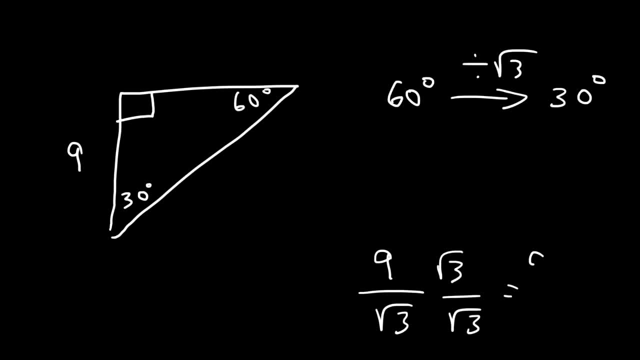 We need to rationalize. So this is going to be 9 square root 3 divided by 3.. And 9 divided by 3 is 3.. So across the 30,, this is going to be 3 square root 3.. 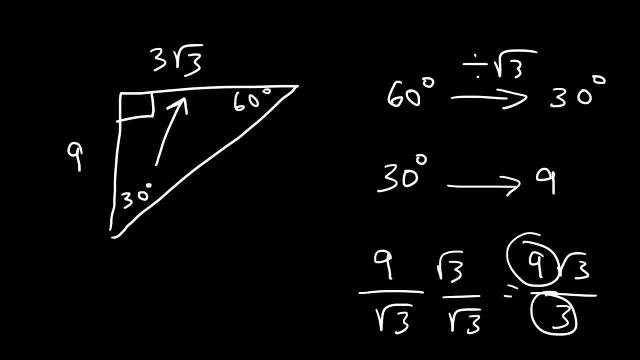 Now, once we have the side across the 30 degree angle, we could find the side across the 90 degree angle by multiplying by 2, since we're looking for a longer side, So we're looking for the hypotenuse. 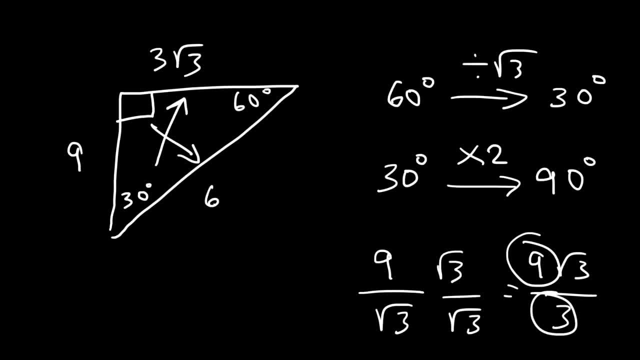 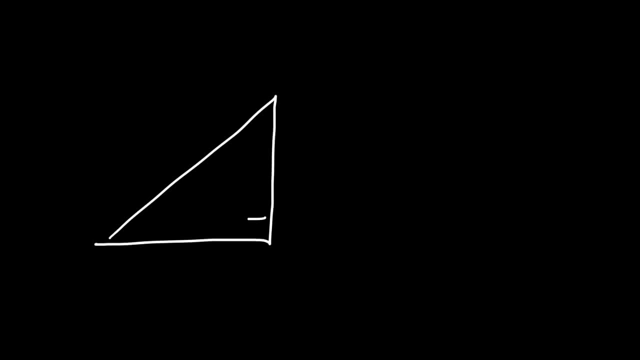 It's going to be this times 2.. 3 times 2 is 6.. So this is going to be 6 times the square root of 3.. And so that's it for that example. Try this one. So let's say we have the side 14, square root 3,. 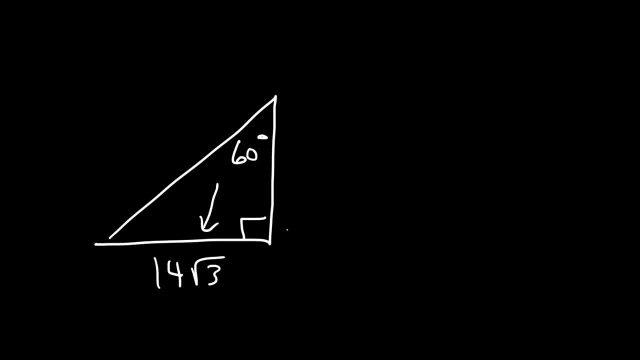 which is across the 60 degree angle. Go ahead and solve this triangle. So once again, let's look for the side across the 30 degree angle. So we need to divide by the square root of 3.. 14 root 3 divided by the square root of 3.. 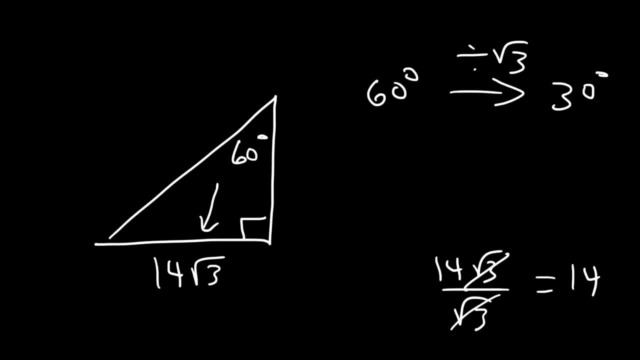 These two will cancel, And this is just going to be 14.. So across the 30 degree angle, the side value is 14.. Now to go from 30 to 90, we know we need to multiply by 2.. 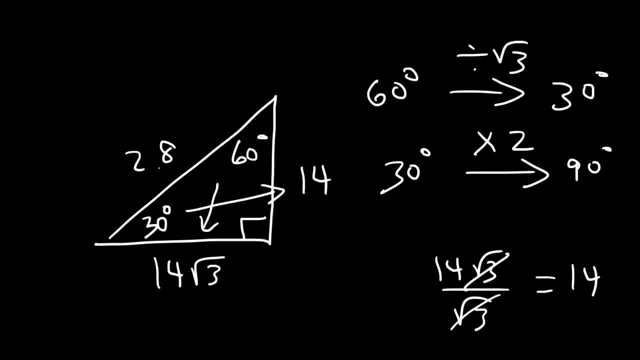 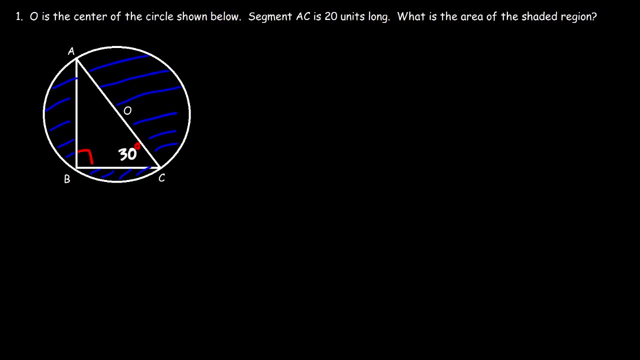 So 14 times 2,, that's 28.. And so that's how you can quickly solve a 30-60-90 right triangle. It's by knowing this information. So here is the typical SAT math question. O is the center of the circle shown below. 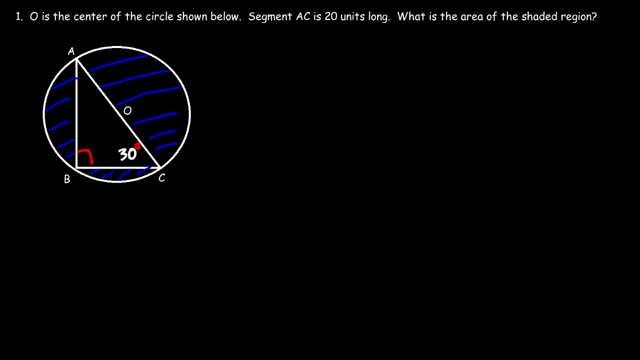 Segment AC is 20 units long. What is the area of the shaded region? In order to find the area of the shaded region, you could pause the video, by the way, if you want to try it yourself. The area of the shaded region is the difference between the area of the large object and the area of the small object. 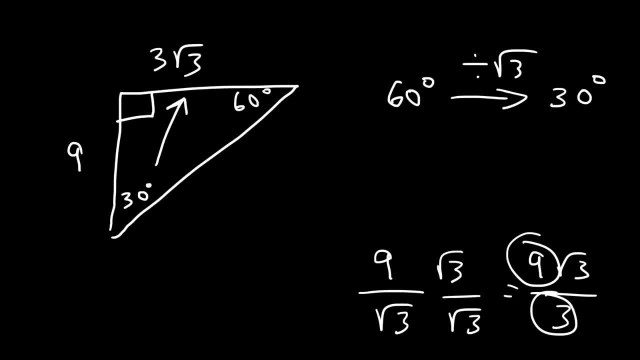 across the 30 this is going to be 3 square root 3 now once we have the side across the 30-degree angle we could find the side across the 90-degree angle by multiplying by 2 since we're looking for a longer side so we're looking for the hypotenuse it's going to be this times 2 3 times 2 is 6 so this is going to be 6 times the square root of 3 and so that's it 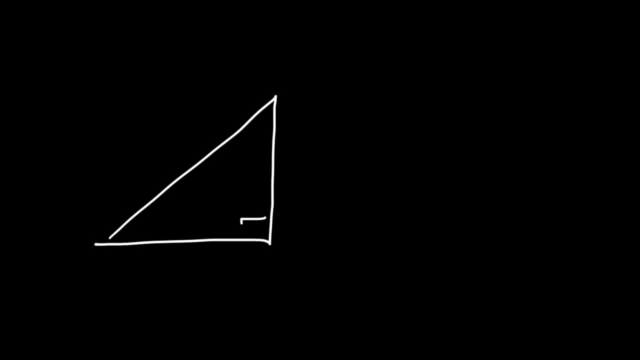 for that example try this one so let's say we have the side 14 square root 3 which is across the 60-degree angle go ahead and solve this triangle so once again let's look for the side across the 30-degree angle so we need to divide by the square root of 3 14 root 3 divided by the square root of 3 these two will cancel and this is just going to be 14 so across the 30-degree angle the side value is 14 now to go from 30 to 90 we know we need to multiply by 2 so 14 times 2 that's 28 and so that's how you can quickly solve a 30 60 90 right triangle it's by knowing this 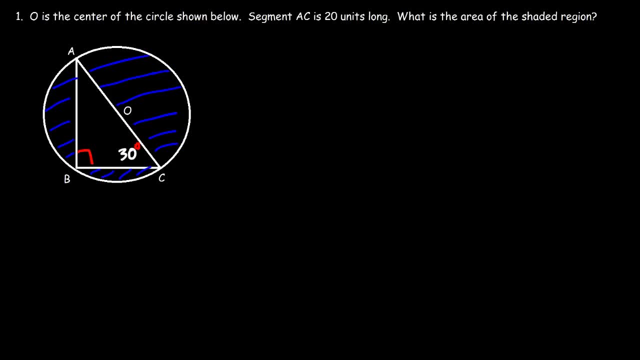 information so here is the typical SAT math question O is the center of the 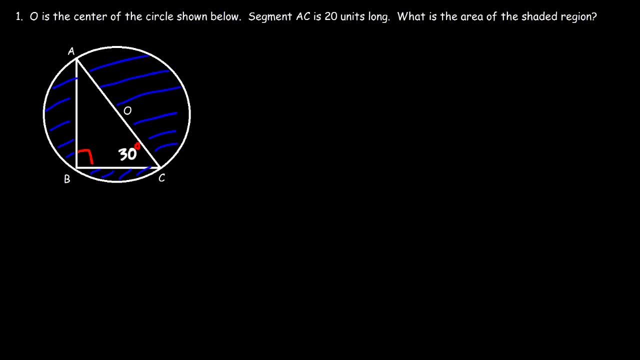 circle shown below. Segment AC is 20 units long. What is the area of the shaded region? In order to find the area of the shaded region, you could pause the video by the way if you want 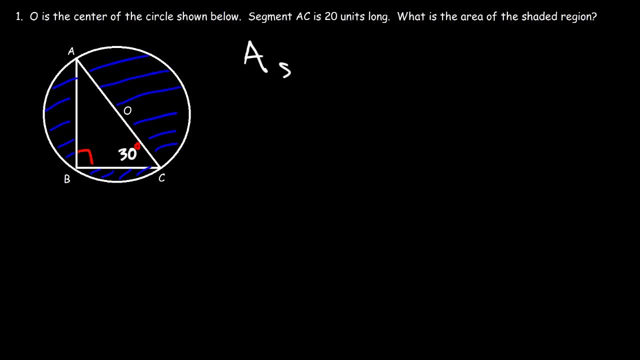 to try it yourself, the area of the shaded region is the difference between the area of the large object and the area of the small object. The large object is the circle, the small object is the triangle. The area of a circle is pi r squared and the area of a triangle, a right triangle, is one half base times height. So right now we have a 30-60-90 triangle. So this is 30 and this is 60. And AC, which is basically the hypotenuse of the triangle, is 20 units long. So we have 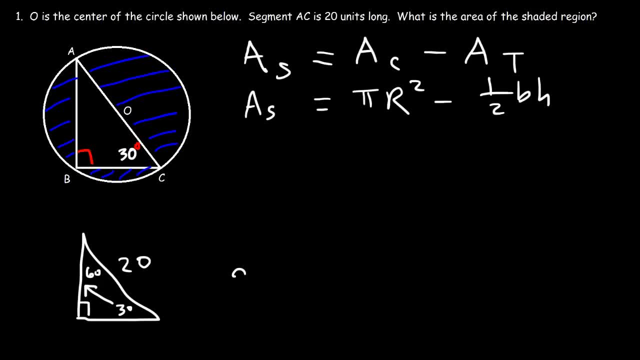 the hypotenuse. To find the side across the 30, so we're going from 90 to 90. 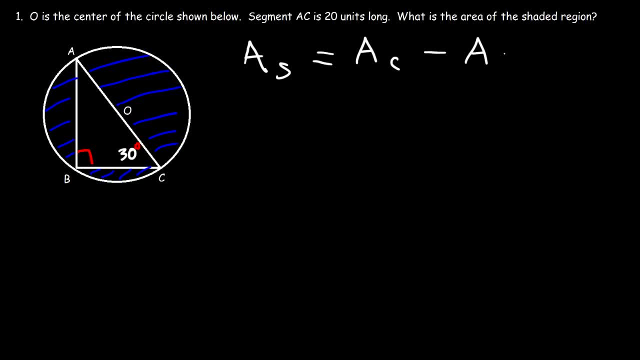 The large object is the circle. The small object is the triangle. The area of the circle is pi r squared And the area of a triangle- a right triangle- is 1 half base times height. So right now we have a 30-60-90 triangle. 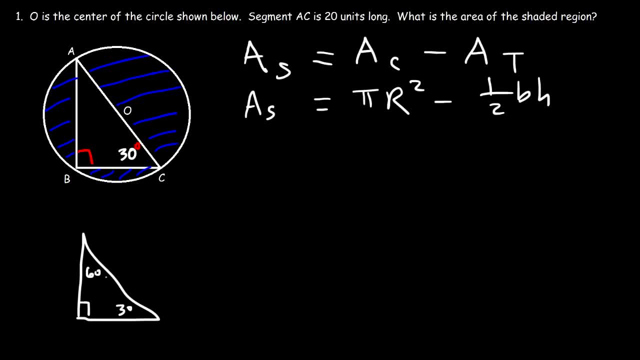 So this is 30 and this is 60. And AC, which is basically the hypotenuse of the triangle, is 20 units long. So we have the hypotenuse To find the side across the 30, so we're going from 90 to 30,. 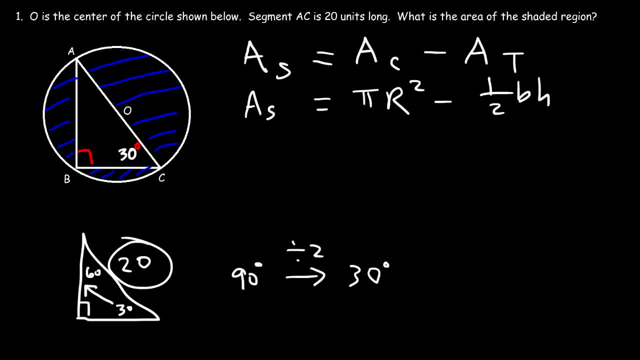 we know we need to divide by 2.. So half of 20 is 10.. So the height of the triangle is 10.. Now to find the side across the 60, so this has to be 60, and granted, the figure may not be drawn to scale, so keep that in mind. 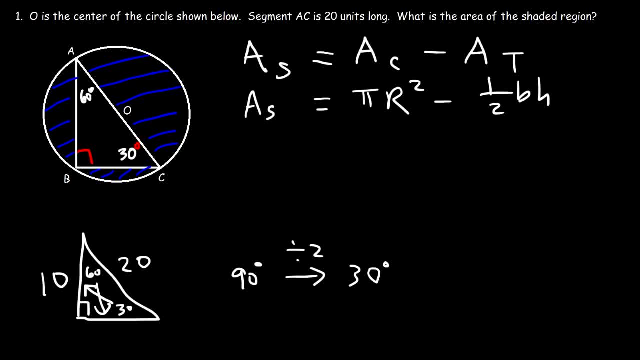 because AB does look longer than BC. To find the side across the 60, we need to go from 30 to 60. So we're looking for a longer side. so we're going to multiply by the square root of 3.. 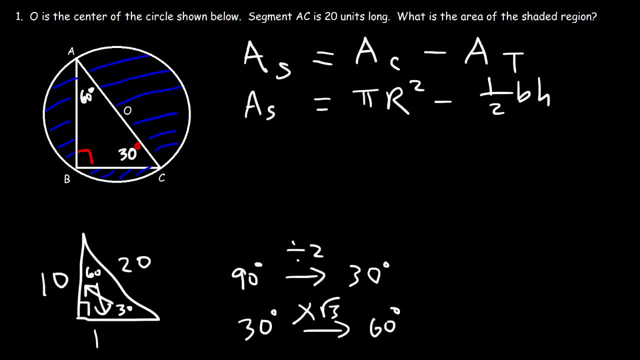 So we need to multiply the side across the 30 by the square root of 3.. So that's 10 root 3.. So now we have the base of the triangle, which is 10 square root 3, and we have the height of the triangle. 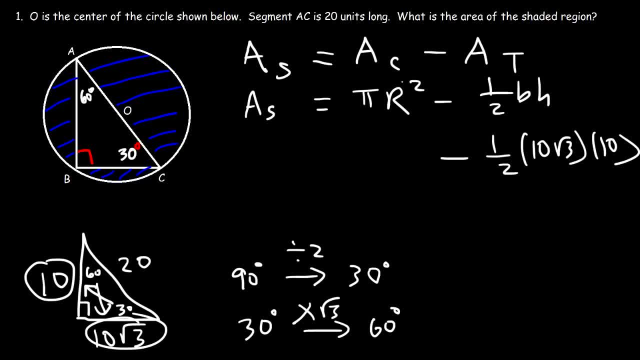 which is 10.. All we need to do is find the radius of the circle. Now, segment AC is the diameter of the circle. because it passes through the center O, The diameter is twice the radius. So if the diameter is 20 units long, 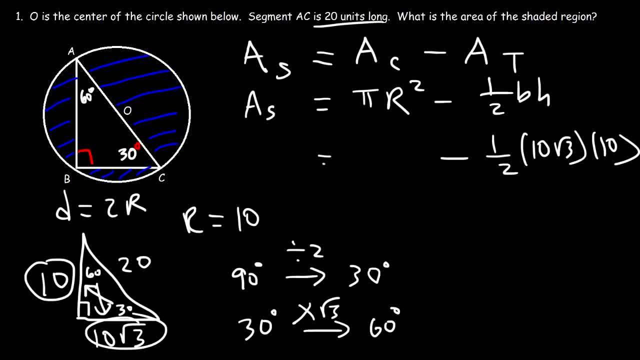 the radius is going to be half of that, So that's 10 units long. So the area of the circle is going to be pi times 10 squared. 10 squared is 100, and 10 times 10 is also 100,. 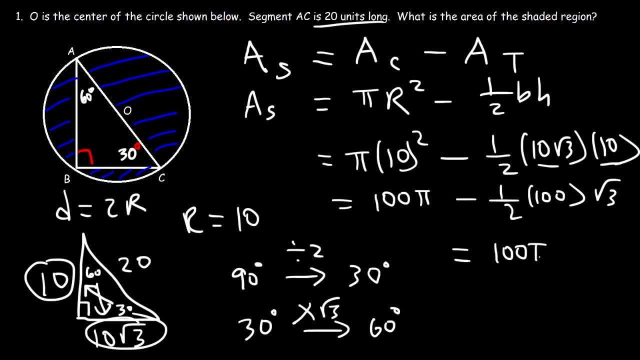 and half of 100 is 50. So the area of the shaded region is 100 pi minus 50 square root 3.. So this is the exact answer. but now let's get the answer as a decimal. So as a decimal. 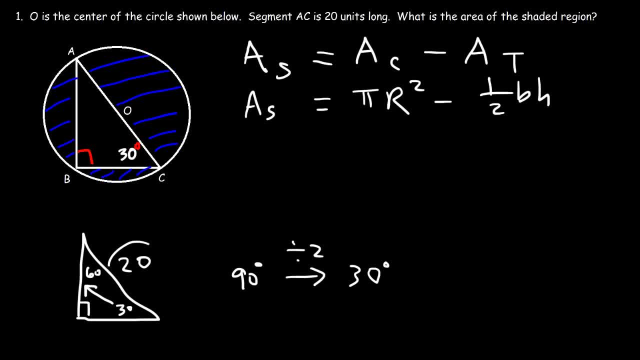 To 30, we know we need to divide by 2. So half of 20 is 10. So the height of the triangle is 10. Now to find the side across the 60, so this has to be 60. And granted, the figure may not be 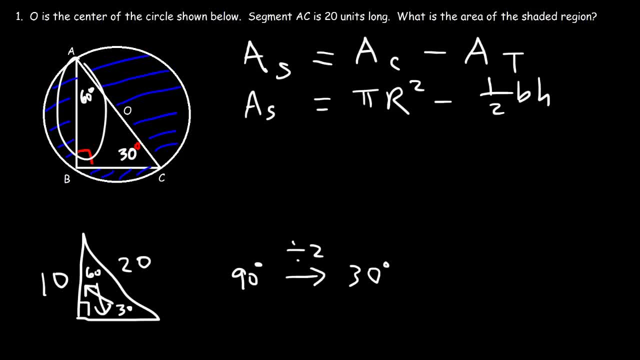 drawn to scale, so keep that in mind because AB does look longer than BC. To find the side across the 60, we need to go from 30 to 60. So we're looking for a longer side, so we're going to multiply by the square root of 3. 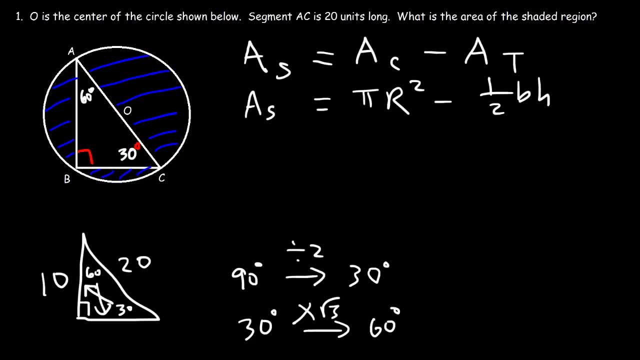 So we need to multiply the side across the 30 by the square root of 3, so that's 10 root 3. So now we have the base of the triangle, which is 10 square root 3. 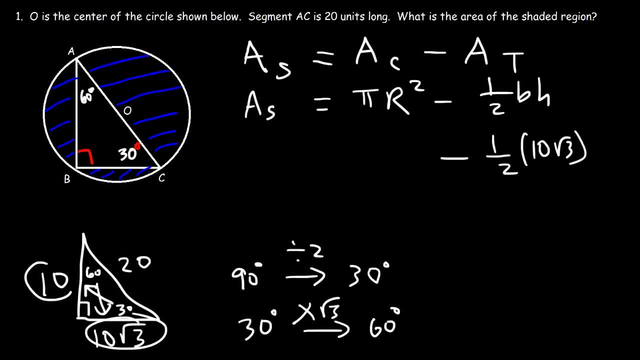 And we have the height of the triangle, which is 10. All we need to do is find the radius of the circle. Now segment AC is the diameter of the circle because it passes through the center O. 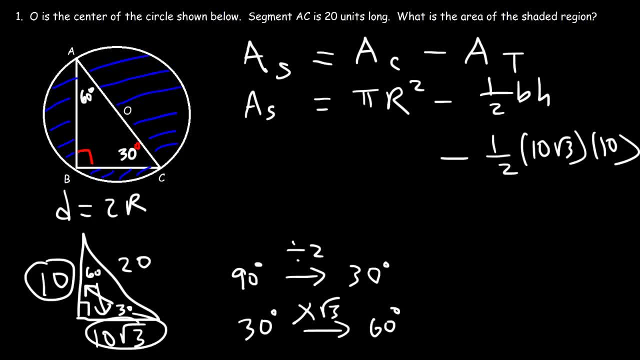 The diameter is twice the radius. So if the diameter is 20 units long, the radius is going to be half of that. It's 10 units long. So the area of the circle is going to be pi times 10 squared. 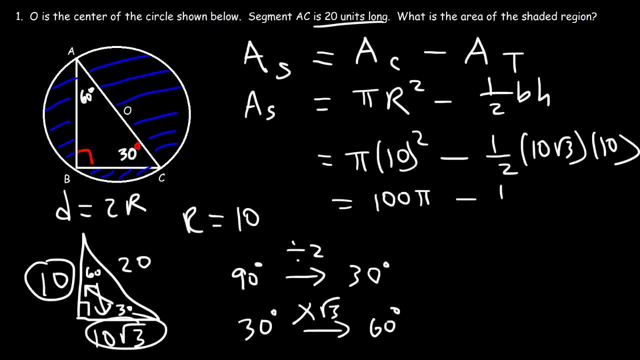 10 squared is 100. And 10 times 10 is also 100. 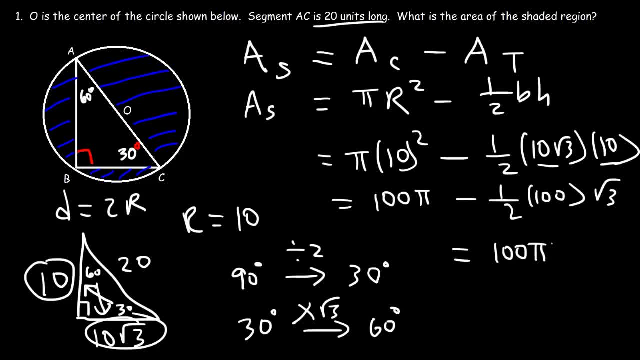 And half of 100 is 50. So the area of the shaded region is 100 pi minus 50 square root 3. So this is the exact answer. But now let's get the answer as a decimal.